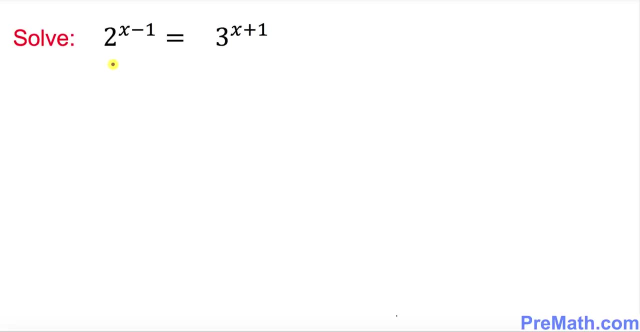 logarithm to solve this problem. so let's go ahead and take a log on both sides. i'm going to put log on the left hand side and log on the right hand side as well, and now we will be using this fact. this is if you have a log of x and you have an exponent m. 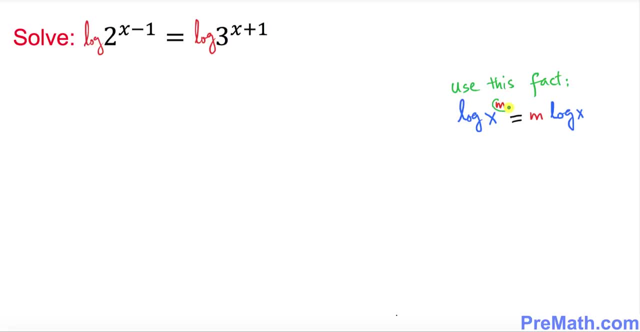 so this is the log of x and you have an exponent m. so this is the log of x and you have an exponent m. this is exponent rule. then what happens to the exponent? you just simply move it to the front. that's all you have to do. so this is the fact that we're going to use to simplify this problem. 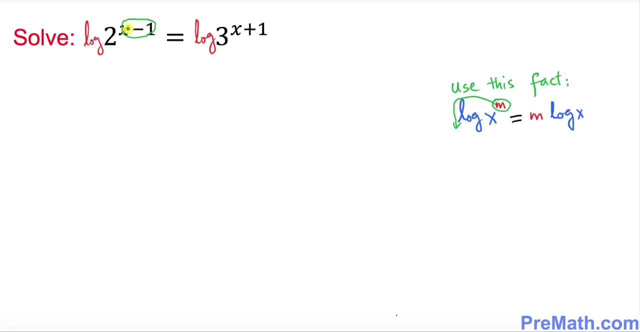 so over here, in our case, on the left hand side, this is our exponent. we're going to move it to the front. likewise, x plus 1 exponent: we're going to move it to the front as well. so then this problem is going to look like x minus 1 times log of 2, equal to x plus 1 times log of 3. let's go. 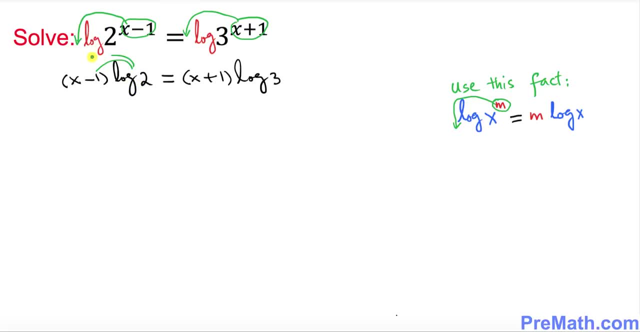 ahead and distribute log of 1 and x likewise over here. so we're going to get x times log of 2 minus 1 times log of 2 is log of 2 and on the right hand side, x times log of 3 plus 1 times log of 3 is. 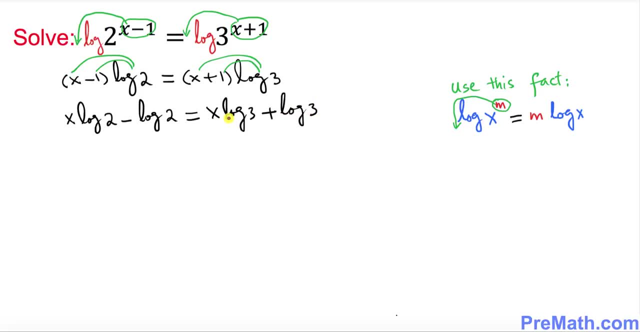 log of 3. now what we want to do is i want you to move this part x log of 3 on the left hand side and this negative log of 2. i want you to move it on the right hand side. so this x log of 2 is: 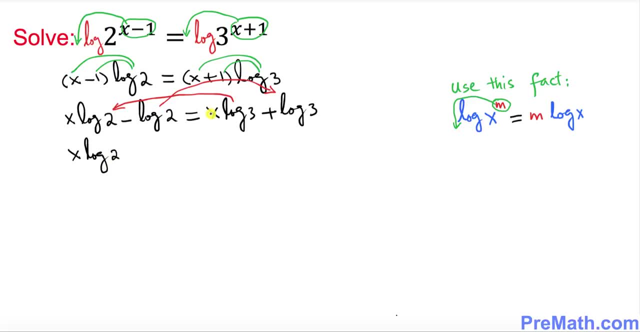 already on the left hand side. just leave it there. and this next, this x log of 3 becomes negative x log of 3, piece of cake equals to. we already have a log of 3 on the right hand side and when you move, negative log of 2 becomes positive log of 2. so far, so good. look at the left hand side. we see x. 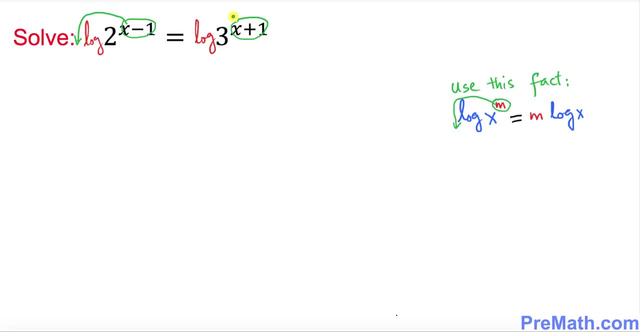 the front. likewise x plus 1 exponent. we're going to move it to the front as well. so then this problem is going to look like x minus 1 times log of 2, equal to x plus 1 times log of 3. let's go. 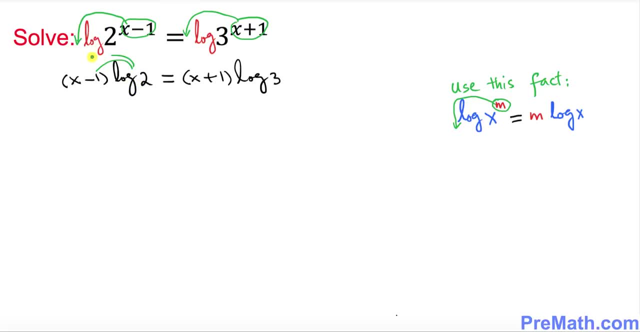 ahead and distribute log of 1 and x likewise over here. so we're going to get x times log of 2 minus 1 times log of 2 is log of 2 and on the right hand side, x times log of 3 plus 1 times log of 3 is. 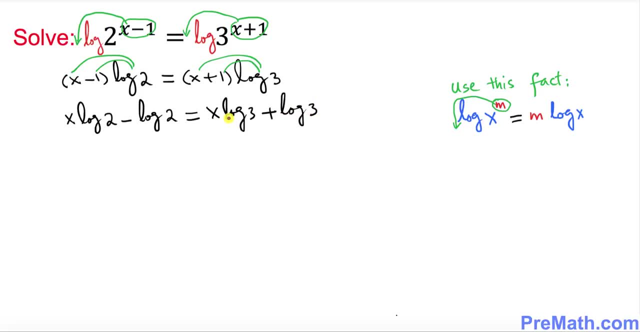 log of 3. now what we want to do is i want you to move this part x log of 3 on the left hand side and this negative log of 2. i want you to move it on the right hand side. so this x log of 2 is: 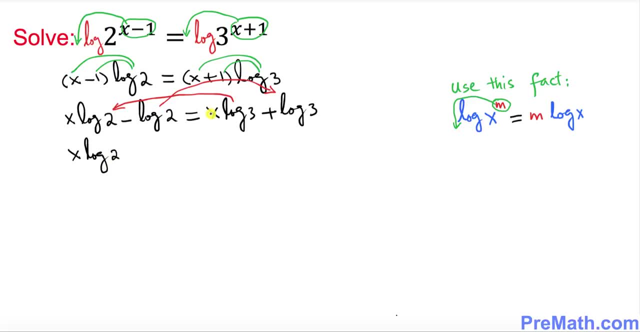 already on the left hand side. just leave it there. and this next, this x log of 3 becomes negative x log of 3, piece of cake equals to. we already have a log of 3 on the right hand side and when you move, negative log of 2 becomes positive log of 2. so far, so good. look at the left hand side. we see x. 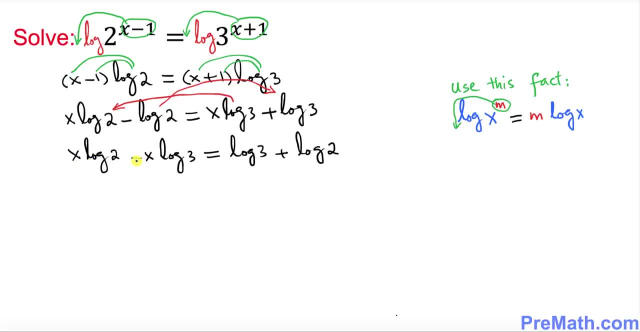 as you can factor out, because x is common. so i can put x outside and you put down log of 2 minus log of 3 equal to log of 3 plus log of 2. now what we want to do is we want to isolate x so that 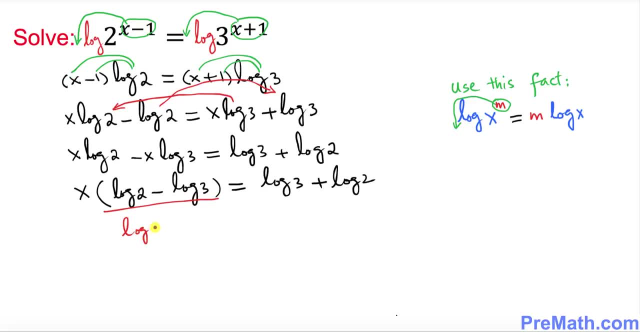 means we're going to be dividing both sides by log of 2 minus log of 3 on this side, and likewise log of 2 minus log of 3 on this side. so this whole thing is gone with this one. so simply we ended up. x equals to: 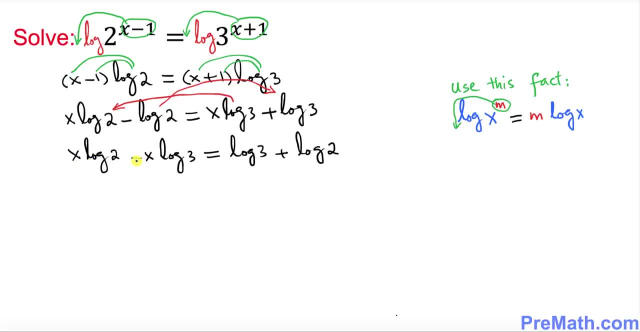 as you can factor out, because x is common. so i can put x outside and you put down log of 2 minus log of 3 equal to log of 3 plus log of 2. now what we want to do is we want to isolate x so that 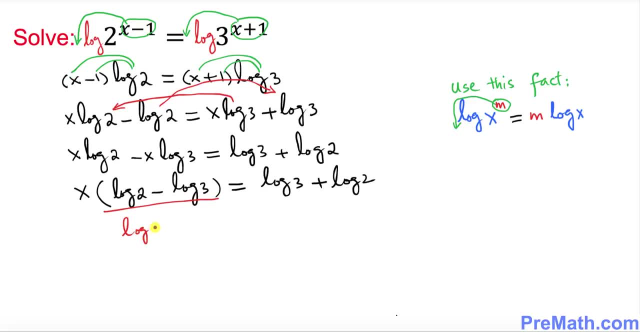 means we're going to be dividing both sides by log of 2 minus log of 3 on this side, and likewise log of 2 minus log of 3 on this side. so this whole thing is gone with this one. so simply we ended up. x equals to: 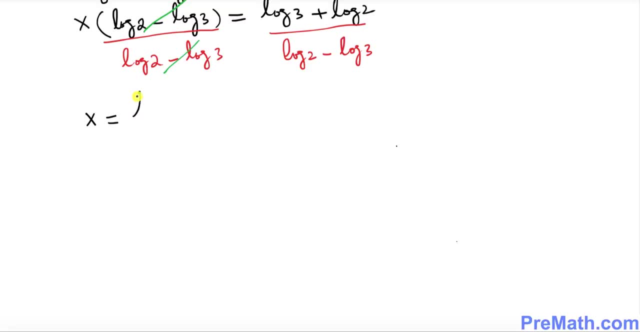 log of 3 plus log of 2, divided by log of 2 minus log of 3. now the next step is use your calculator and figure out log of 2 and log of 3, and here i have already figured out. log of 2 is approximately: 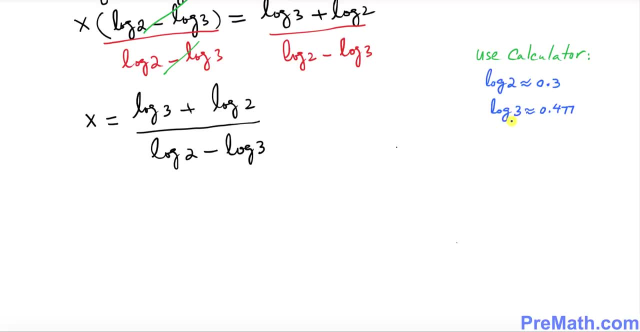 equal to 0.3 and log of 3 is approximately equal to 0.477, so let's plug it in those values right up here. so x equal to log of 3 is 0.477 plus log of 2 is 0.477. 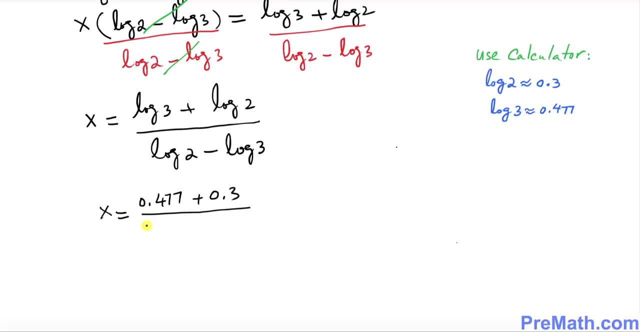 divided by log of 2 is 0.3 minus 0.4, and if you simplify these ones, that's going to give you, on the top, 0.777 divided by negative 0.177, And if you divide it, that's going to give you approximately equal to negative 4.4..